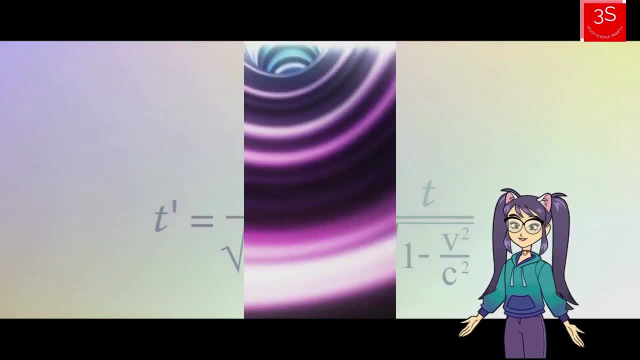 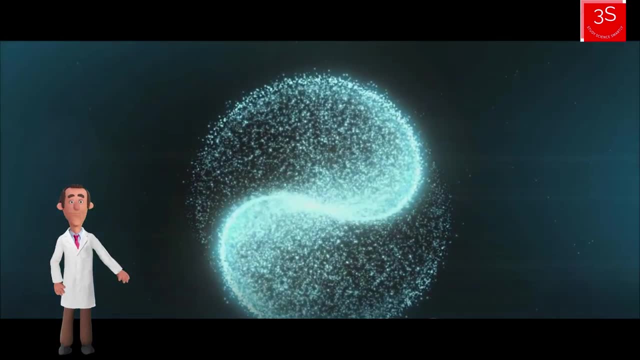 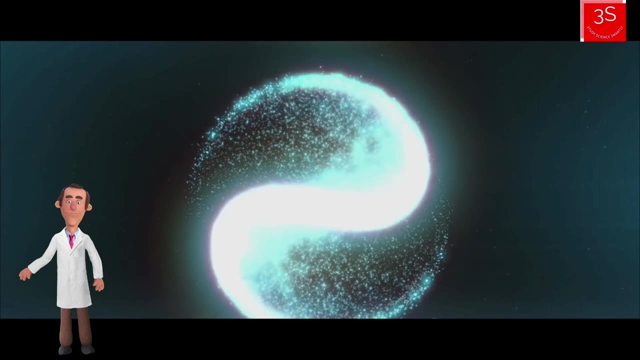 at speeds close to the speed of light. Enter Einstein and his revolutionary theory of relativity. Photons, being massless particles, defy the classical understanding of momentum. However, in the quantum realm, things get interesting. Thanks to their wave-particle duality, photons exhibit 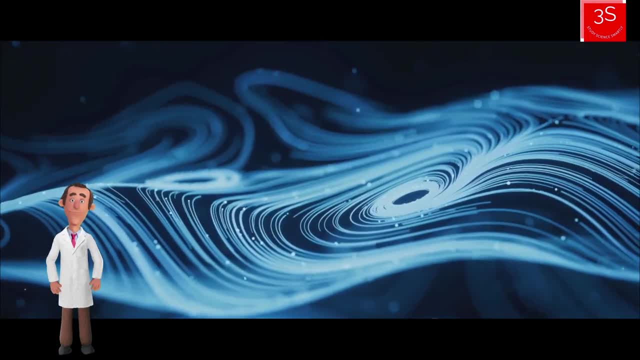 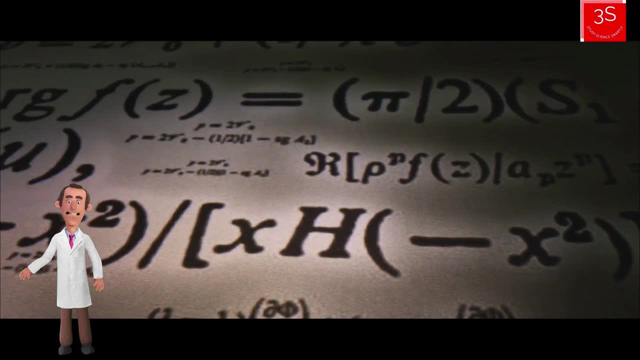 some particle-like and wave-like properties. As photons travel with the speed of light, their momentum is defined in a little different manner. Now let's unlock the secret formula for momentum of light. Let's start with the secret formula for momentum of light. Let's start with. 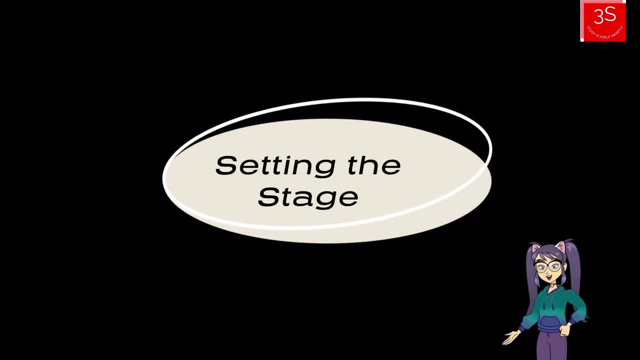 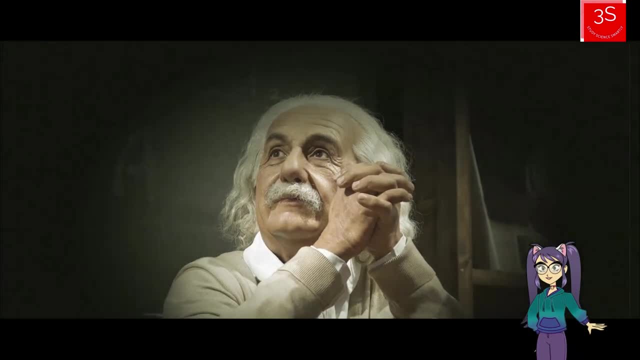 the secret formula for momentum of light. Let's start with the secret formula for momentum of light. The momentum of photons, Planck's constant, denoted as h, plays a crucial role. The relativistic mass m becomes infinite as the velocity of the body approaches the speed of light. The momentum of a 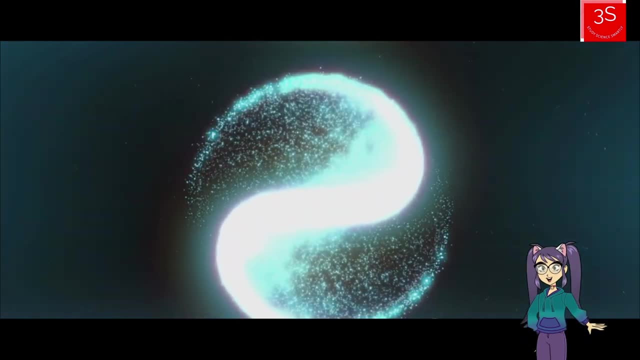 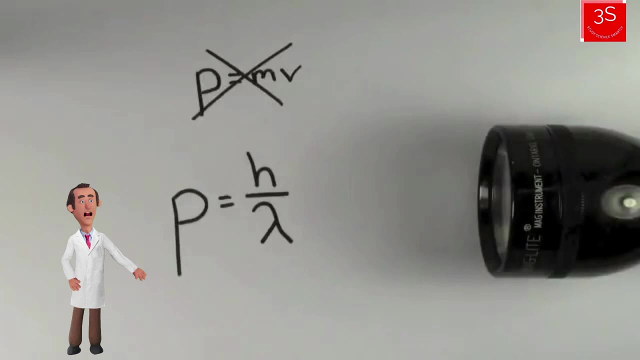 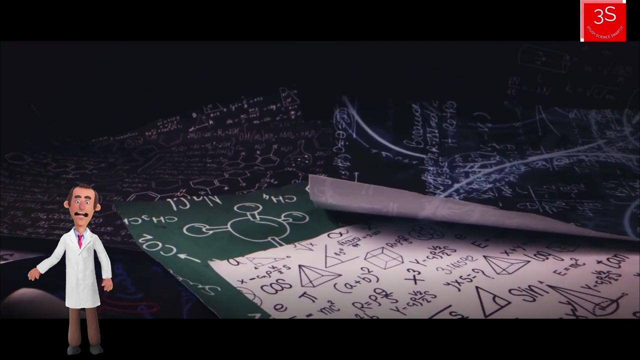 photon, which moves with a speed equal to that of light, is given by the equation shown in picture. This formula, which says p equals h over lambda, where lambda is the wavelength of the photon, is a planned equation. photon represents the correct picture of the scenario here. here's the kicker. even. 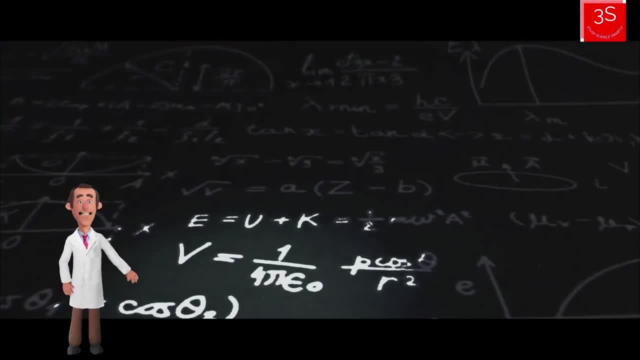 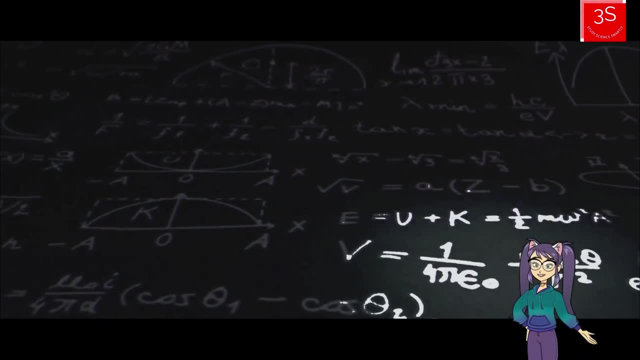 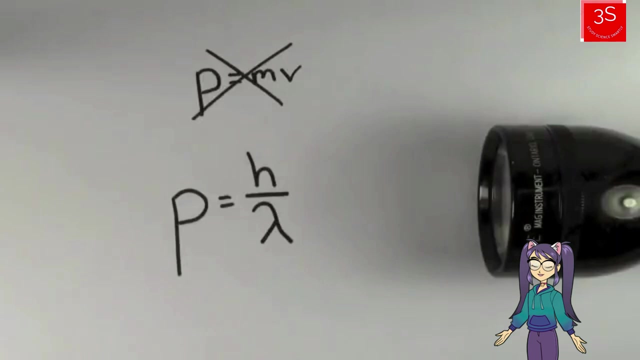 though photons have zero rest mass, they carry momentum because of their energy and wavelength. from the formula it is quite clear that shorter the wavelength, the higher the momentum. this is the unseen force that propels light through space and enable us to see various objects of this world in special. 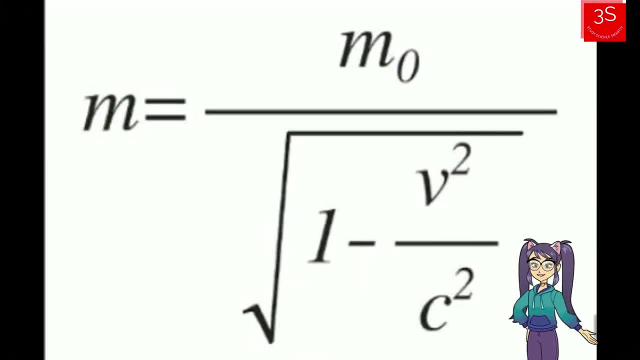 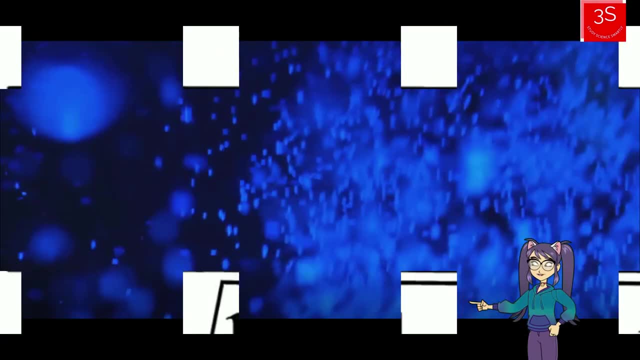 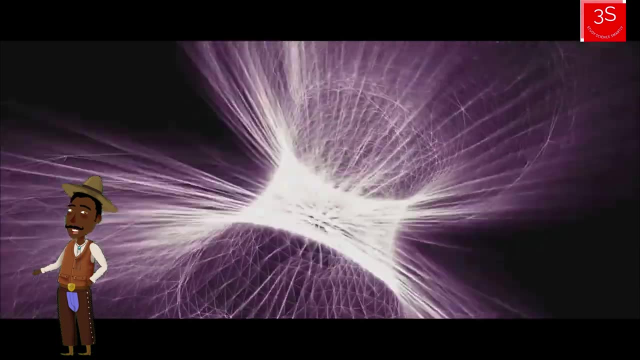 relativity. the relativistic mass is given by M sewers gamma times the rest mass of object. here gamma is the Lorentz factor. the Lorentz factor shows the formulas for the Lorentz transformation and expresses the relativistic mass, momentum and energy. it also appears in the equations that describe how the 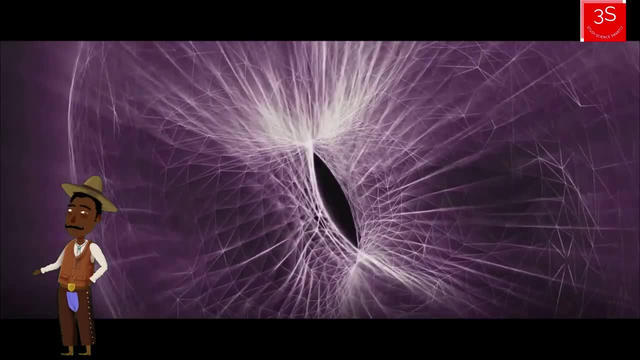 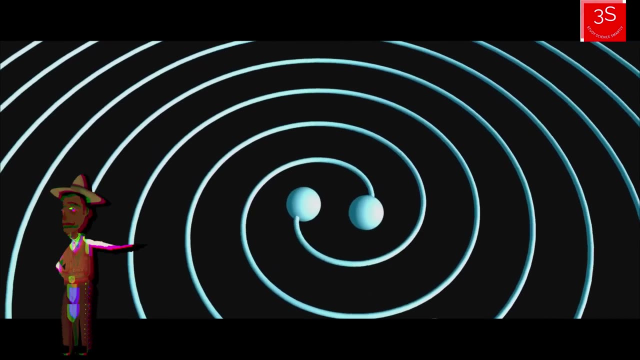 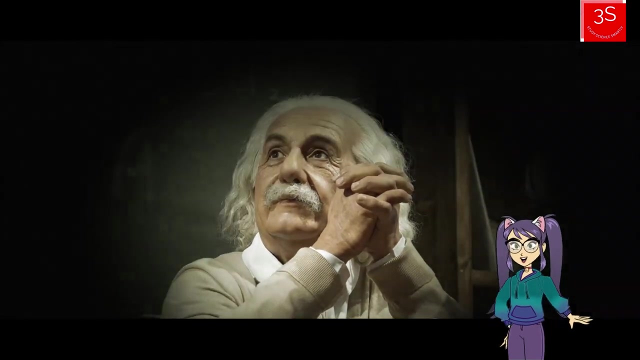 electromagnetic fields transform due to motion of an observer. it means that the unusual behavior due to special relativity. it means that the unusual behavior due to special relativity increases with speed. this concept is a beautiful manifestation of Einstein's theory of relativity. the energy of a photon tied to its frequency results in: